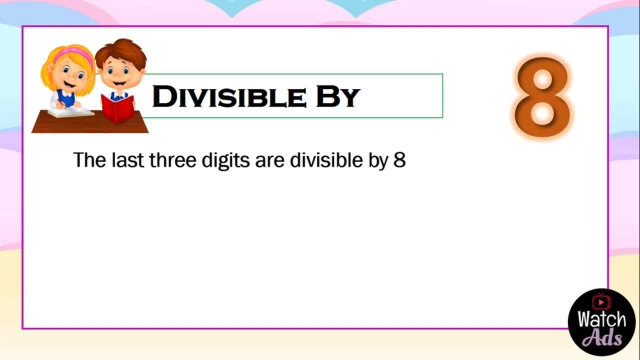 I haven't found a shortcut for this method. I have composed my own and original method. This is my method of testing the divisibility by eight. The first condition to test the visibility by eight is it should be an even number. Let's have our first example: 8371. 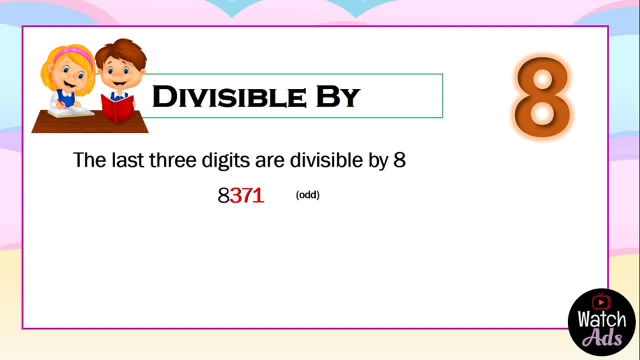 is an odd number, which means that it is not divisible by eight. Now for our next example. we will be needing again our table of four or the multiples of four as our side note. And then our example is 1794.. Now our test says that the last three digits should be: 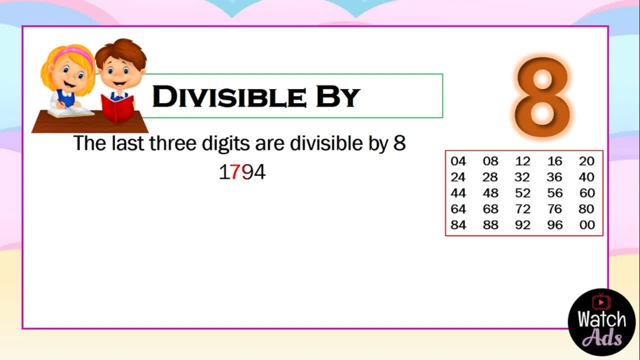 divisible by eight, And the last three digits are 794.. Check if it is odd, or even It is even Now we can proceed with the test. I am going to offer you two methods for this. By the way, both methods will still give you the. 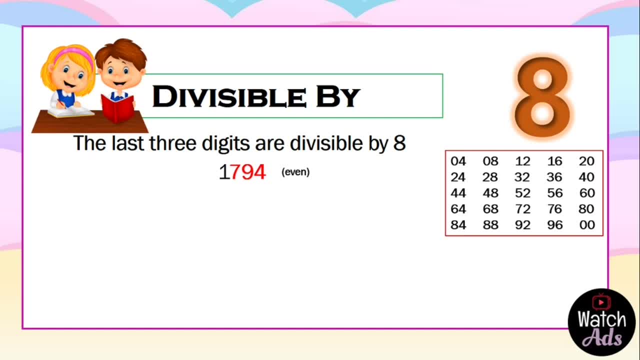 same answer. It is either a yes, it is divisible, or a no, it is not divisible. For our first method, let's have 794, since we are talking about the last three digits. Then we will have again magic numbers: 200,, 400,, 600, and 800.. Now I will tell you that these four numbers 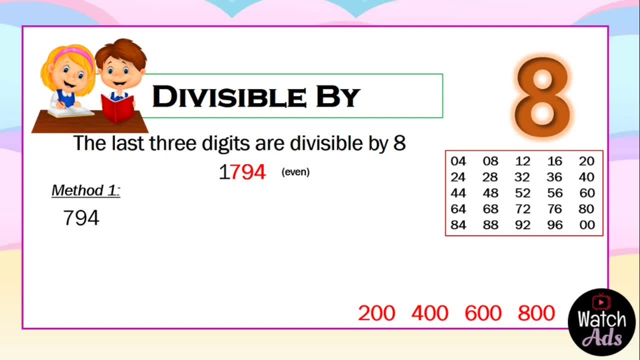 are exactly divisible by eight. Now again we choose which is the largest number that we can subtract from 794, and that is 600.. 794 less 600, because 600 is divisible by eight, The answer is 1794.. Now we take the last digit, four, and divide it by two. The answer is two. And then we 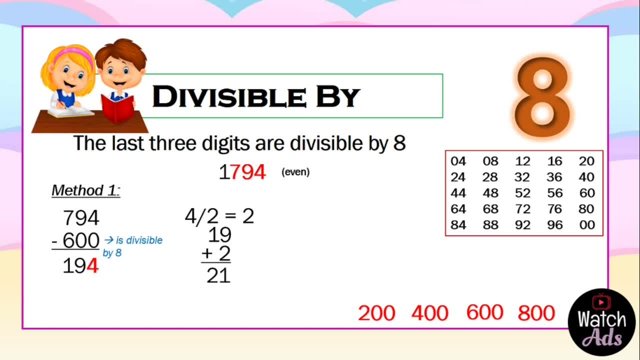 add it to 90. The answer is 21.. We check if 21 is divisible by four. 21 is not divisible by four, which means that 1794 is not divisible by four. Let's see our second method. For our second method again, we take the last three digits and then we check our magic. 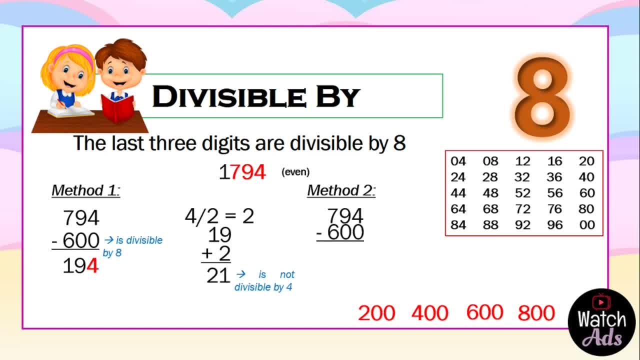 numbers, It is still 600.. 794 less 600 is equal to 194, because we know that 600 is divisible by eight. Next, you think of a number that is divisible by eight. Maybe you will think first of 8,, 16,, 20,, 21,, 22,, 23,, 24,, 25,, 26,, 27,, 28,, 29,, 30,, 31,, 32,, 33,, 34,, 35,, 36,, 37,, 38,. 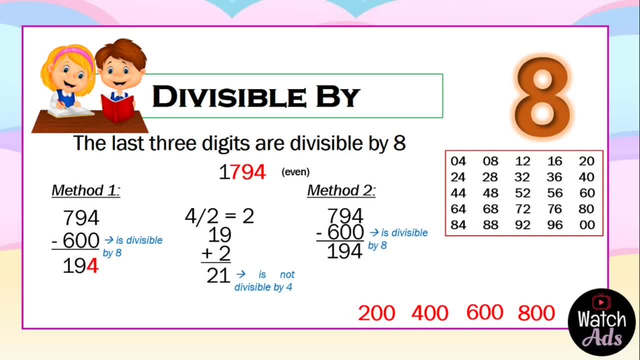 32,, 37,, 38,, 32 to the universities 24 to 20,, 29,, 30,, 64,, 30,, Sinnn and Nick. So 78 minus 74, um It gives 18.. 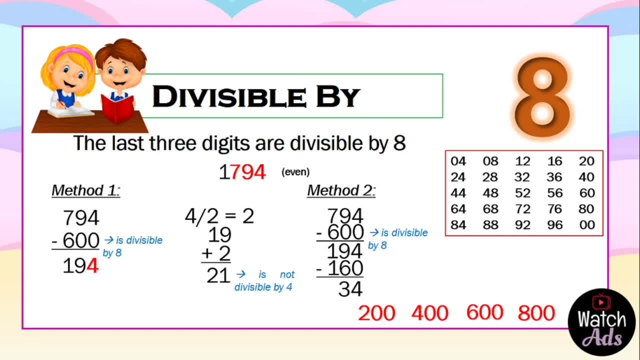 I advise that you use either 80 or 160.. You can also use 160, because 80, multiplied seguir siendo 8 x 10, gives 160.. 194 minus 160 is equal to 34.. And we know that 34 is not divisible by four. Now don't. 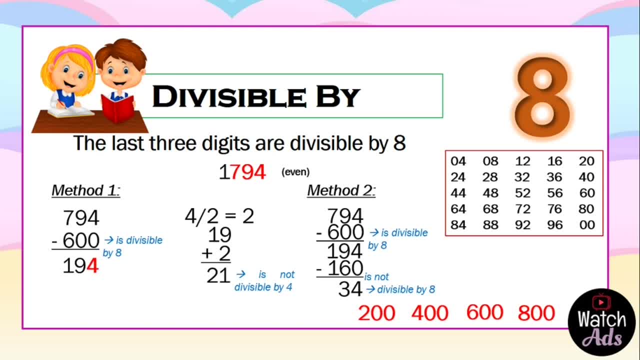 worry, if you subtracted 80 from 194, and then again you subtract it, It should always n Simplify 1,2,1.. subtracted another 80 from 194, because it will still give you the same answer, that is, 34 and 34. 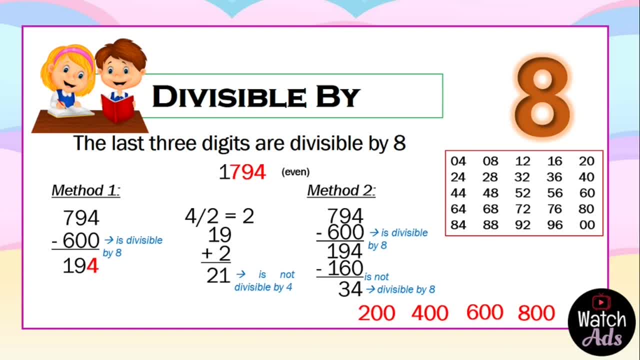 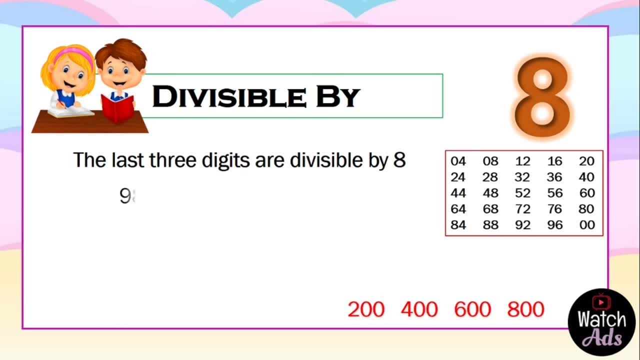 is not divisible by 8, which means that 1794 is not divisible by 8. let's have another example. that is 9816. first we check if it is an even number. and yes, it is an even number. let's take the last three digits, that is 816, and then check the magic numbers. which fits, that is 800, 816 less. 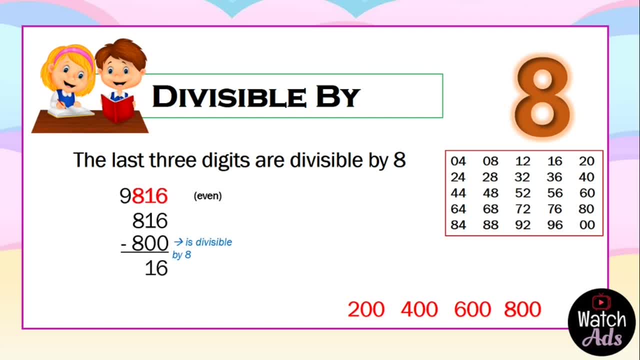 800 gives us 16, and we know that 16 is divisible by 8. but if you still want to proceed and check our first method, we just divide 6 by 2, it gives us 3 plus 1, and 4 is divisible by 4, which means that 9816 is divisible by 8. let's have another example.